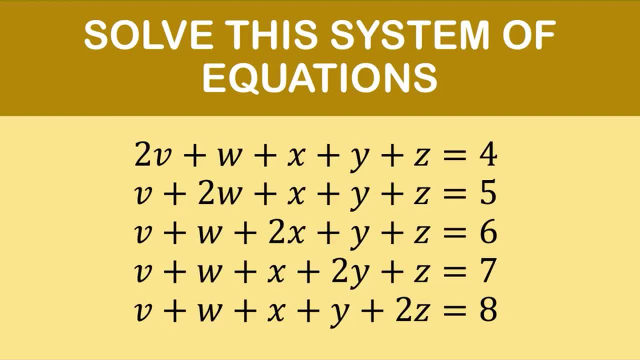 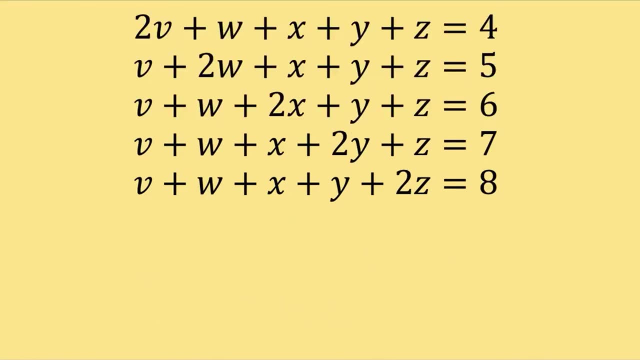 Hi, this is Lando Asistan. In this video, I'm going to show you how to solve this special case of systems of five equations in five unknowns. Let's begin Solve these systems of five equations in five unknowns. This is a special case. To begin our solution, let's call the first equation as: 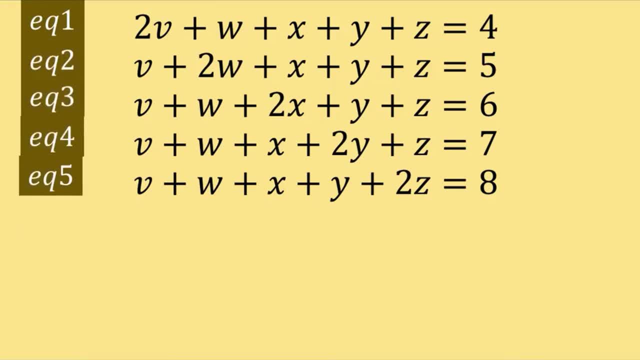 equation 1, the second equation 2, and 3,, 4, and 5 respectively. If you're going to add all these equations vertically like this, let's add 2v plus v plus b plus v plus b In the first column. 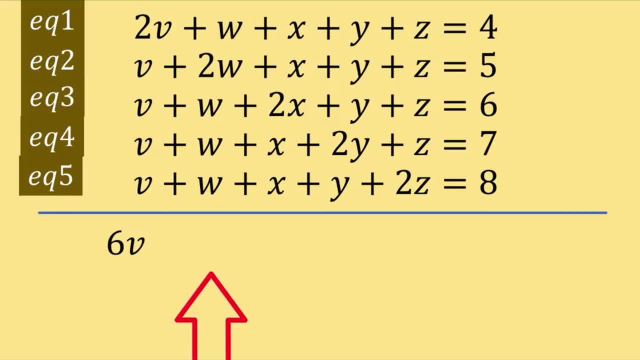 we got 6v. Let's add also all the terms At the second column to get 6w. The third column is added to 6x, The fourth column is added to 6y And the last column of the left side of the equation is added to. 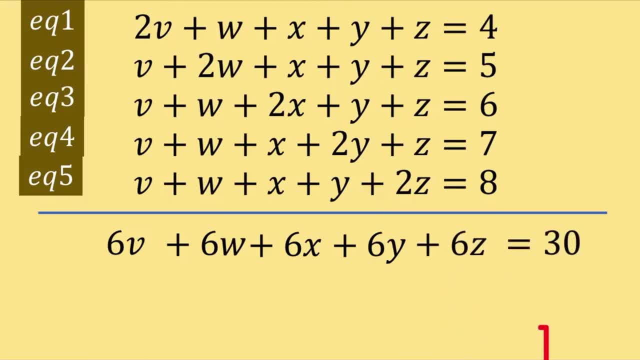 6z Equals the sum of the right side, which is 30.. Notice that 6 is a common factor, so we can factor that out And we arrive at six times the quantity v plus w plus x, plus y plus z equals 30.. 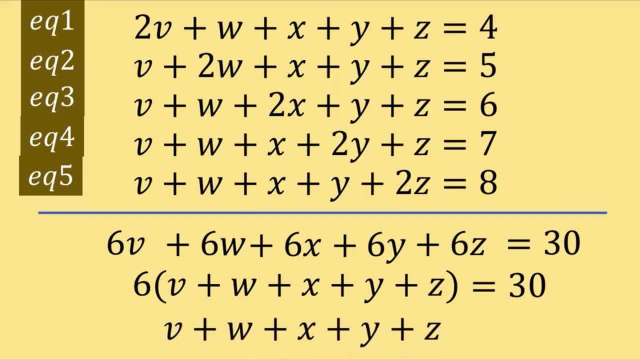 And dividing both sides by 6, we arrive at v plus w plus x plus y plus z equals 30 divided by 6, which is 5.. Now, let's remember this value: The sum of all these 5 variables is equal to 5.. Now let's. 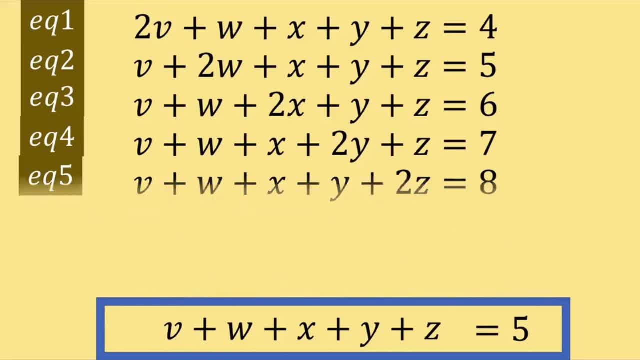 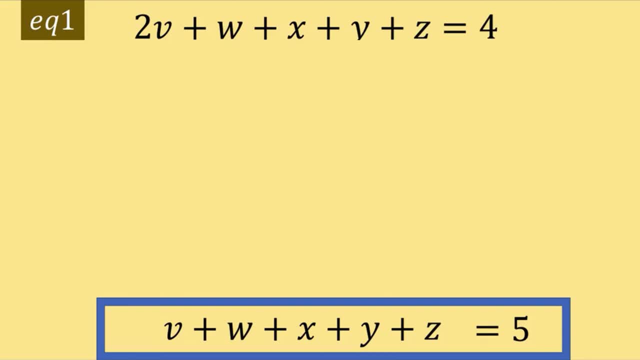 focus on equation number 1 and these results that we arrive at. So we have this equation 1 at the top and we have this value of the 5 variables equals 5 at the bottom. Let's write equation 1 in such a way that this result we have at the bottom can be grouped together like this We can: 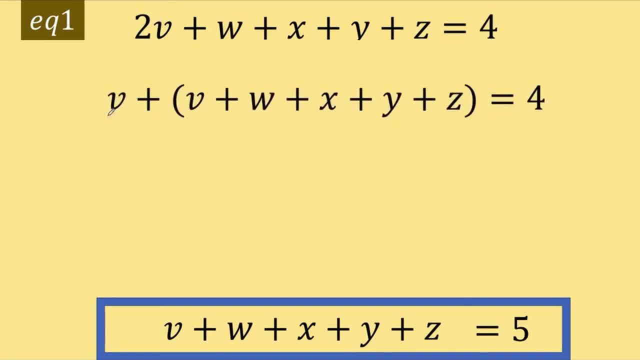 split this 2v as v plus v. So the 2v is now this: v plus b. that is equal to this. And we just copied w plus x plus y plus z. Then copy: the right side equals 4.. But we know the value of this sum. 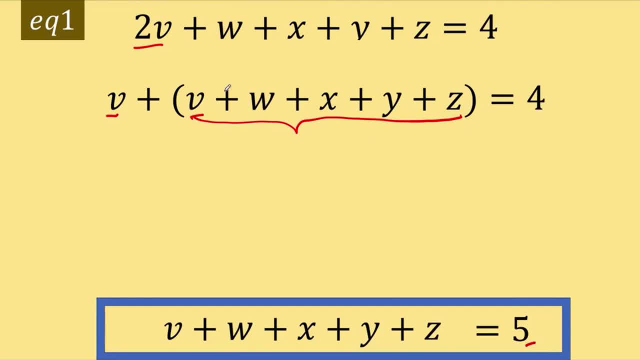 that is equal to this 5.. So, therefore, we just have to copy the v tax and replace this sum by 5, because that's the result that we arrive at, And then copy equals 4.. And finally, we arrive at: v equals 4 minus 5,, which is negative 1.. 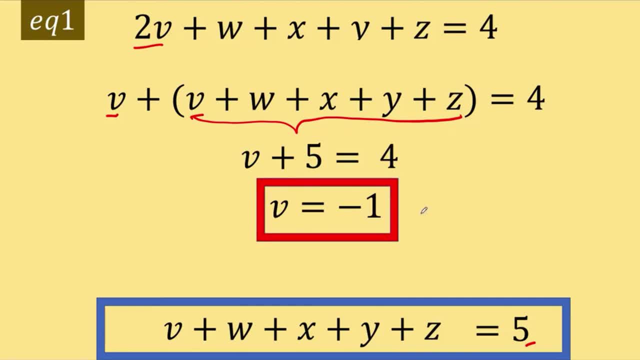 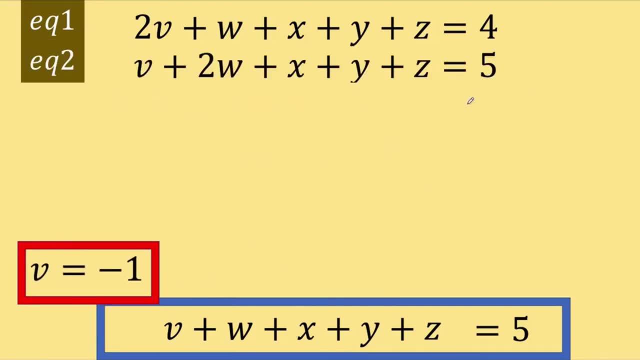 So we now have the value of v, and that is equal to negative 1. Let's put that aside. Next, let's look at equation number 2.. This is equation number 2. And let's reorganize again the terms in such a way that this sum is grouped together. 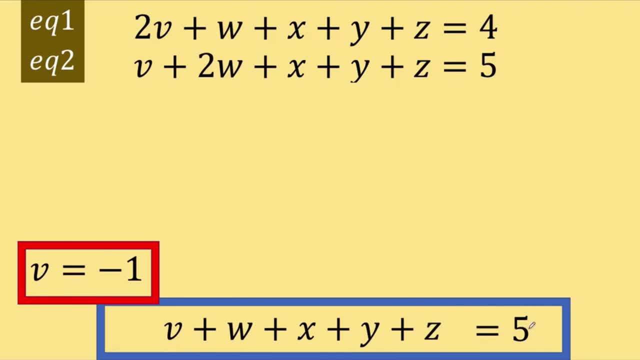 because we know the value of that is 5.. So let's do it this way: Split this 2w as w plus w, and then copy the v plus x plus y plus z, and that's equal to 5.. But again, this is equal to 5, so we have w plus 5 equals 5, which gives us w equals 0. 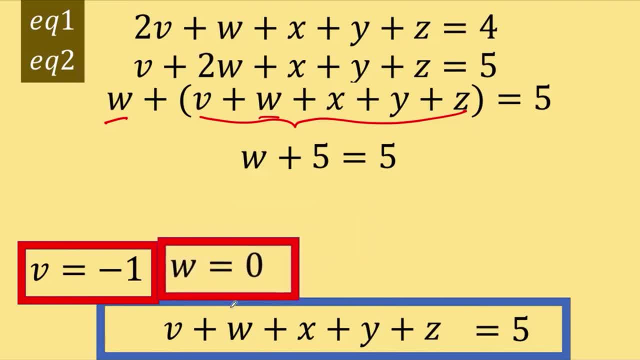 So we now have the value of w, and let's put this aside. Then let's go to equation number 3.. This was equation number 3 in the given, and let's split this 2x as x plus x, again like this: 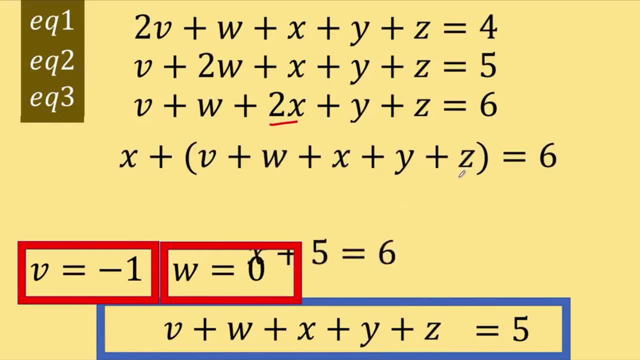 And this part inside the parenthesis is equal to 5, and so we have: x plus 5 equals 6, or x is equal to 6 minus 5 equals 1.. So the value of x is 1.. Let's put that aside also. 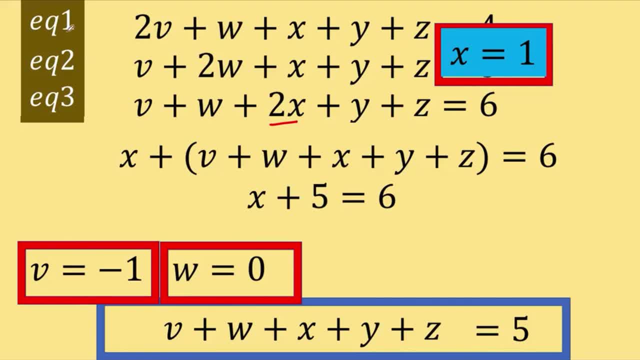 So far, we now have three results here by using equations 1,, 2, and 3.. Now we need more space, so let's put this value. Let's put this value here at the right. Let's visit equation number 4.. 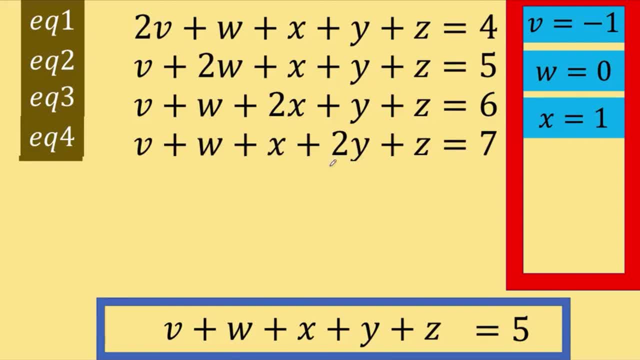 This is our equation number 4, and we split again this 2y as y plus y to arrive at this, And this sum, inside the parenthesis, is equal to 5, so we have y plus 5 equals 7,, which gives us y is equal to 2.. 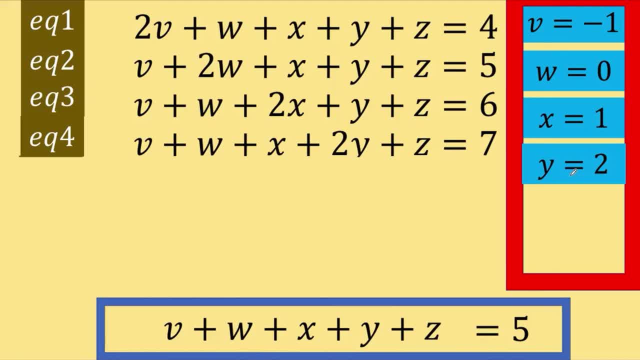 So y is equal to 2.. Then, lastly, go to equation number 5. Split this 2c as z plus c to arrive at this. This sum, inside the parenthesis, is equal to 5.. So we have z plus c. 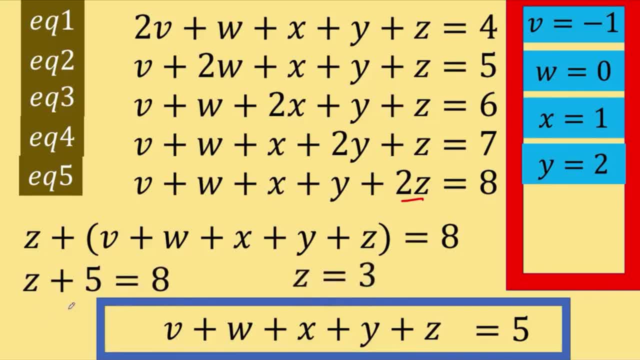 z plus 5 equals 8, or z is equal to 8 minus 5,, which is equal to 3,, and that is the value of z. So at this point we now have all the values of the variables: v equals negative 1,, w equals 0,, x equals positive 1,, y equals 2, and z equals 3.. 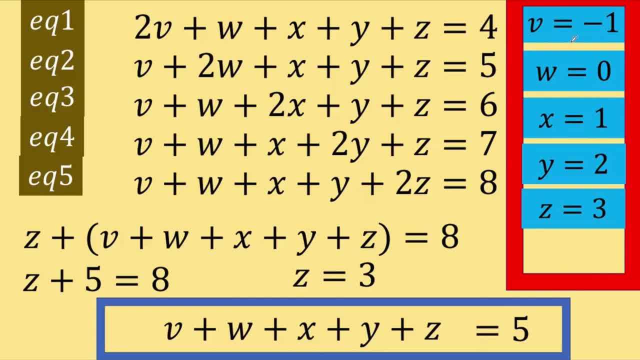 Now to check if this is correct. we can substitute any of these values to any of these five equations and we should be able to come up with a correct equation. Let's just check with one of these equations. Let's choose equation number 3..